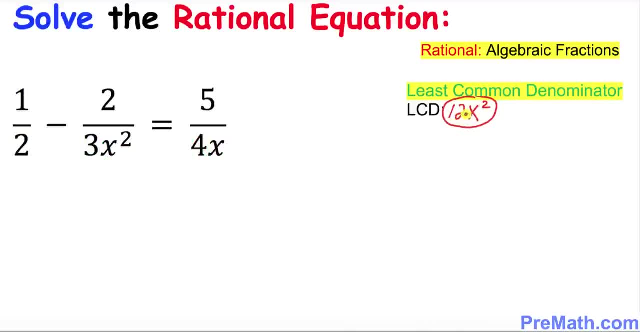 So the next step is: I want you to multiply this 12 x square, the least common denominator across the board. over here, I want to put down 12 x square on the top of the first fraction, and then 12 x square on the second term, and then 12 x square on the third term. 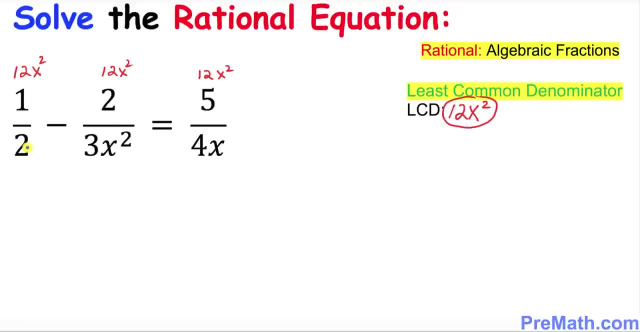 I just multiplied it across the board. Let's simplify this thing. So this 2. 2 goes into 12 six times. So this simply becomes: I want you to just put down 1, this 1, just whatever, 1 times 6x square minus, and then over here you can look at this thing. 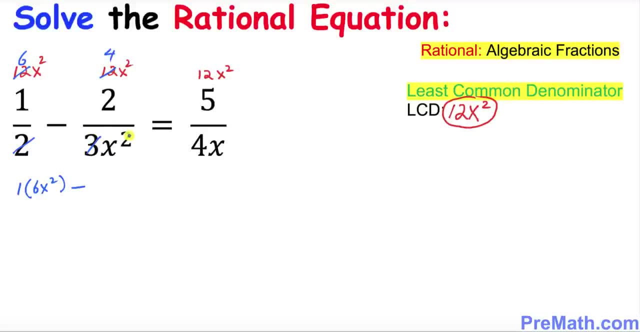 3 goes into 12 four times, and this x square and this x square. they cancel each other out. So we got Negative 2 times this 4.. You just put it down Equals to Same thing we're going to do. 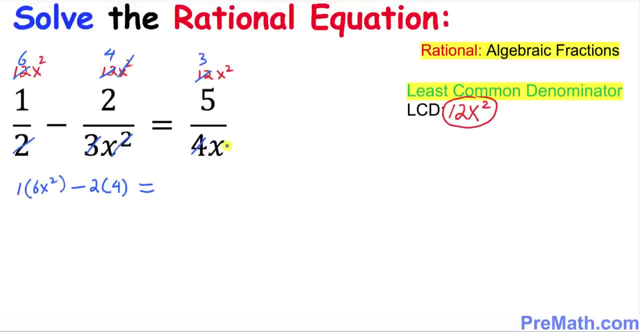 4 divides into 12. three times This 1x cancelled to this x square, We simply ended up with x, So we got simply 5 times 3x. So let's simplify this thing: 1 times 6x square is going to be simply 6x square minus 8.. 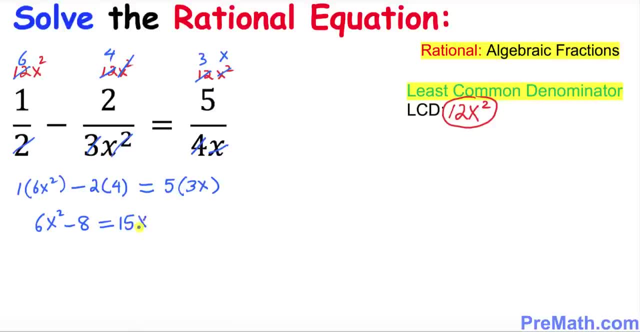 Equals to 15x. I want you to move this 15x on this side, So this simply becomes 6x square. When you move this positive 15x, this become negative 15x- and we already got negative 8 over here- equal to 0.. 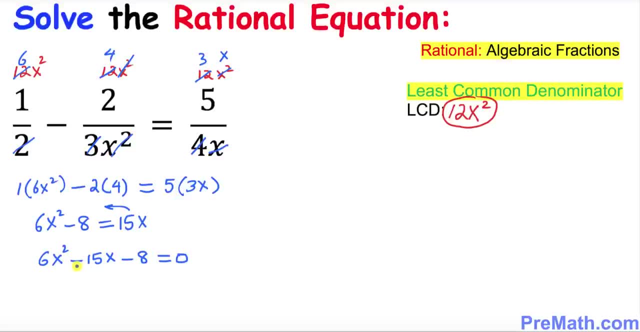 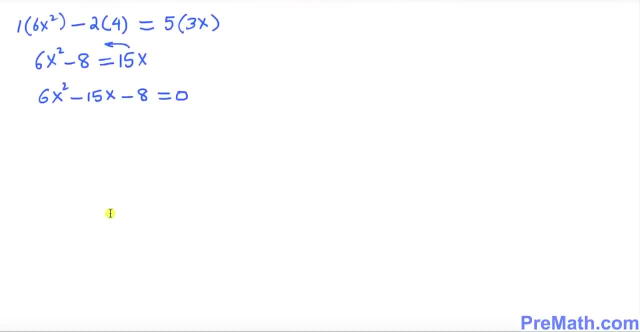 So, as you can see, this is a quadratic equation And we want to solve For this one, for x, And now we're going to be applying this quadratic formula, As you can see over here, where our coefficient a is 6, b is negative 15 and c is negative 8..